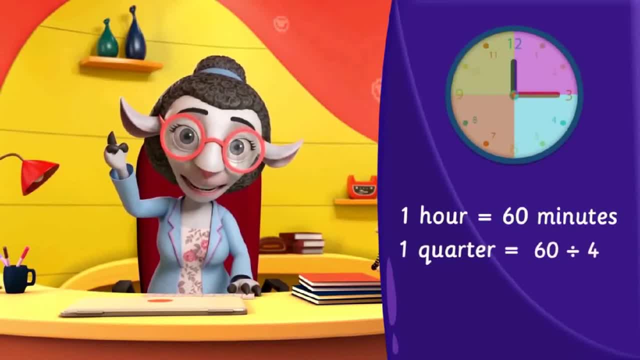 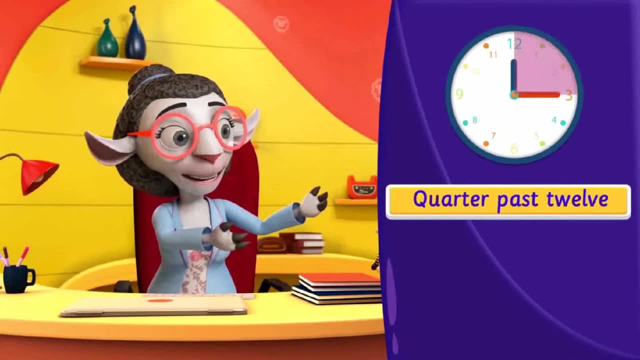 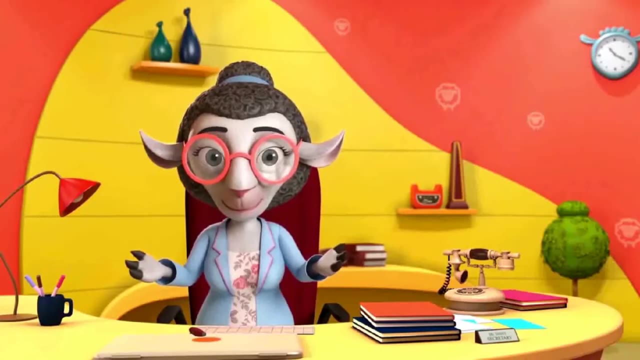 Since an hour is 60 minutes, one quarter is equal to 15 minutes, So we can say that quarter past 12 is 15 minutes past 12 o'clock. This means it's 12.15.. So 12.15 and quarter past 12 both mean the same thing. 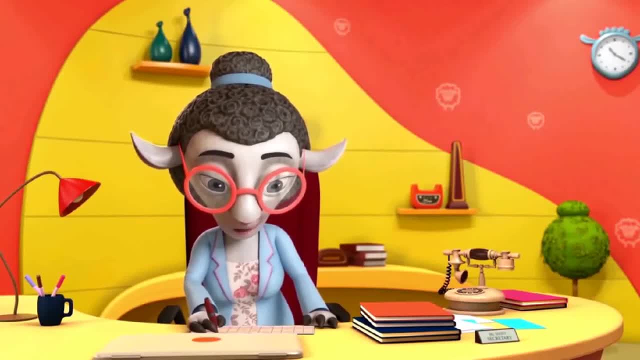 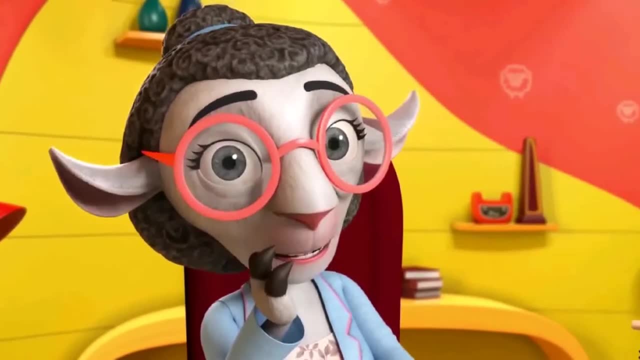 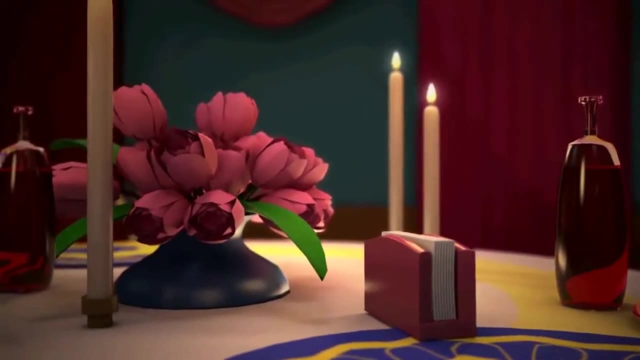 It's in the afternoon, of course, So let's write 12.15 pm in this blank. Great, He says it's for work, but I think they're going out for lunch. There will be candles, flowers, good food. 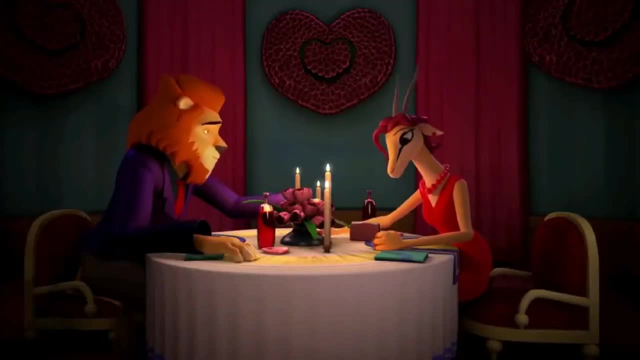 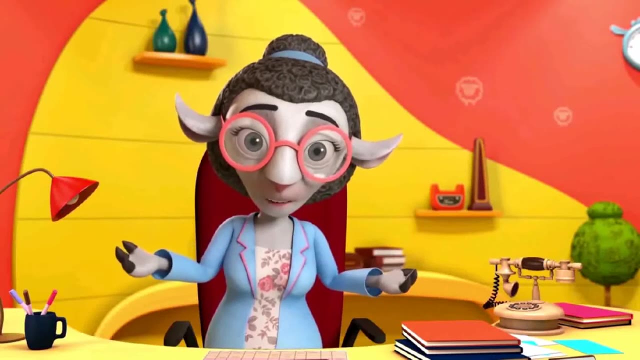 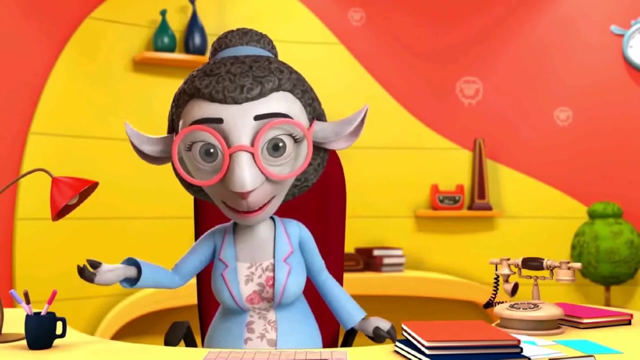 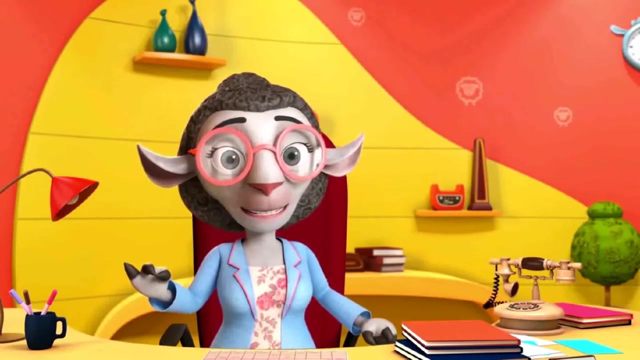 Oh, Ahem, but you didn't hear this from me. Now let's move on to the next day and complete the timetable. Mr Johnny has to attend Mr and Mrs Fly's wedding anniversary at 10.45.. How do we write 10.45 am in words? 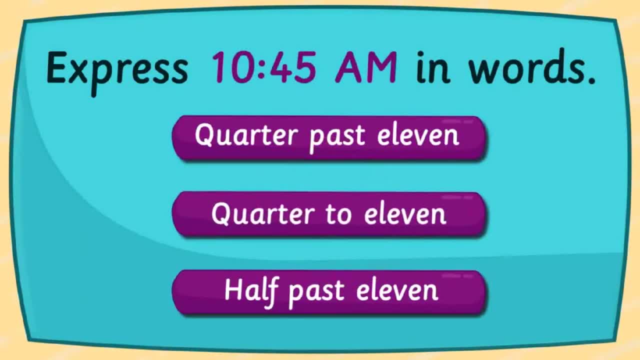 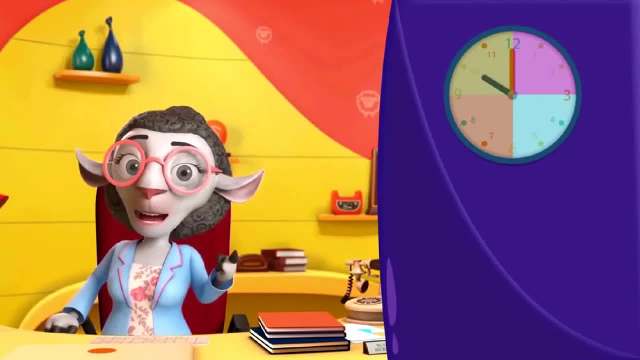 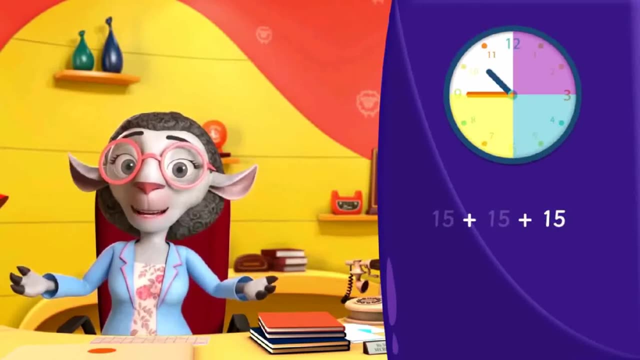 Tap on what you think is the right answer. Brilliant, Let's see. Since one hour has four quarters, we can say that we are three quarters past 10.. That is 15 plus 15 plus 15 minutes past 10,, which is 45 minutes. 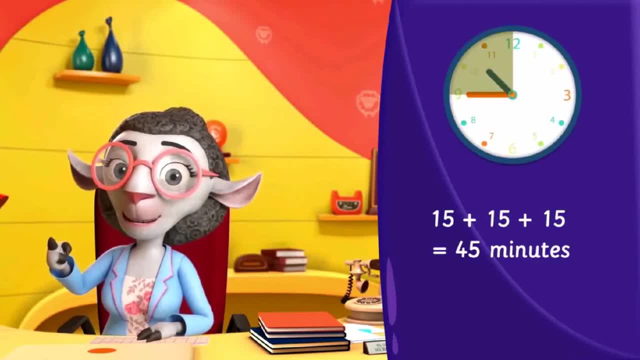 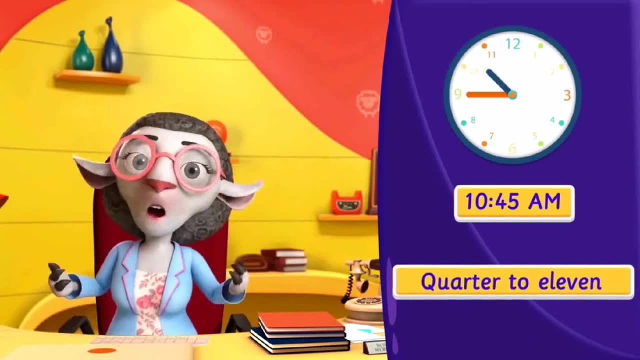 But you can also think of this as just one quarter or 15 minutes away from 11 o'clock, So we can write 10.45 as quarter to 11.. I'll have to remind Mr and Mrs Fly that I'm not going to write 10.45.. 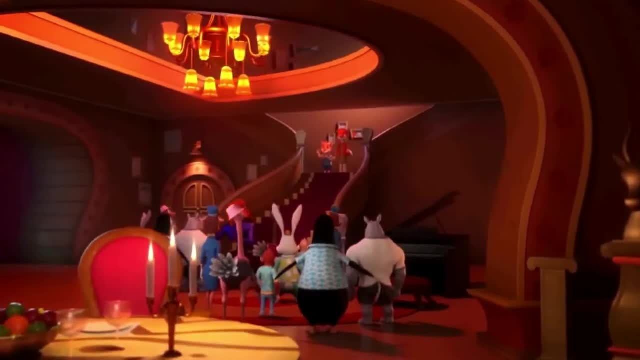 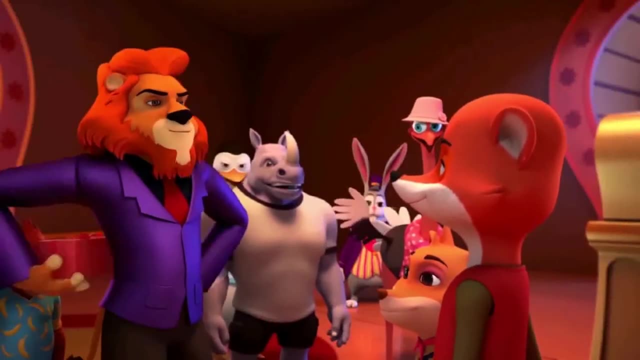 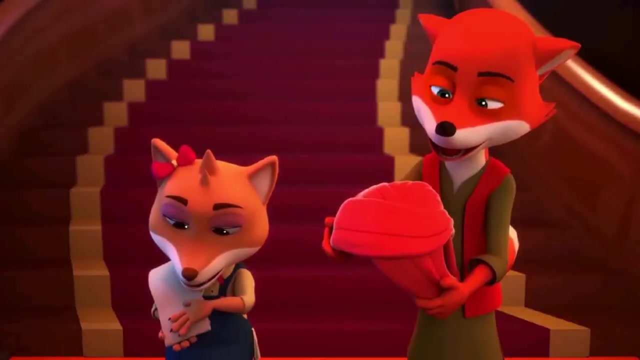 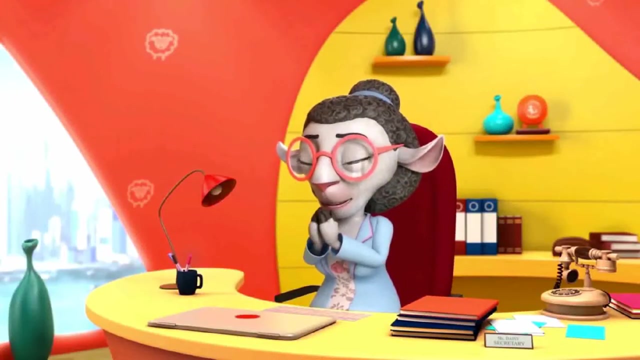 So we need to challenge Mr and Mrs Fly. The drawing's a game-changer, I know It'll try to describe something: I'm gonna be danced. I'm excited, I'm so excited. Thank you, Hello, Mr and Mrs Fly. 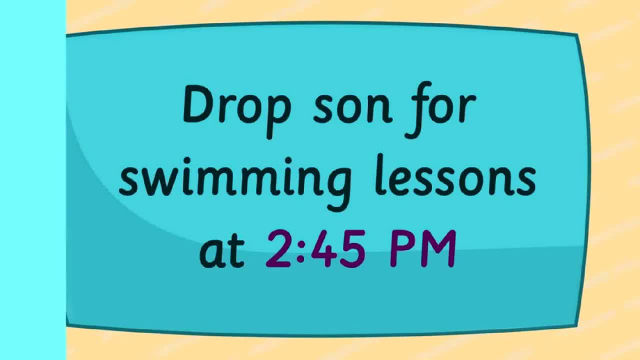 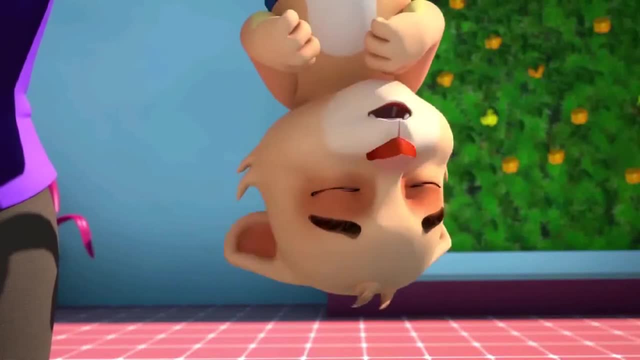 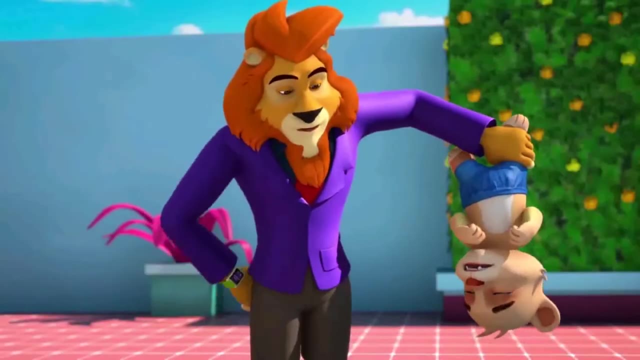 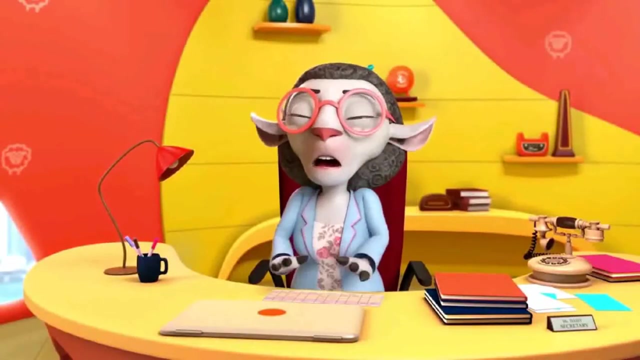 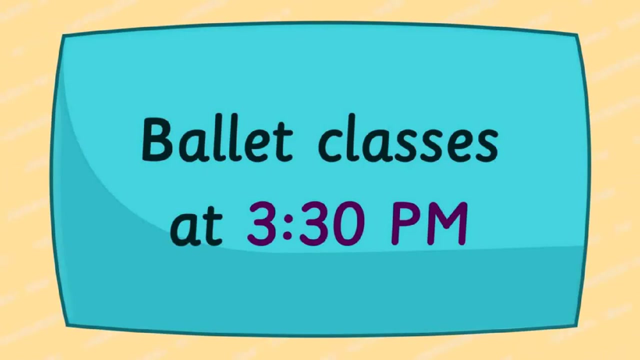 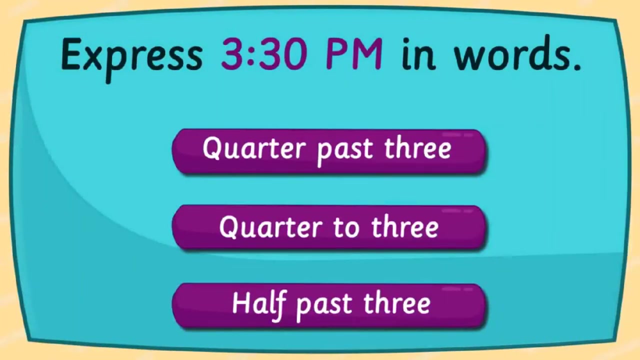 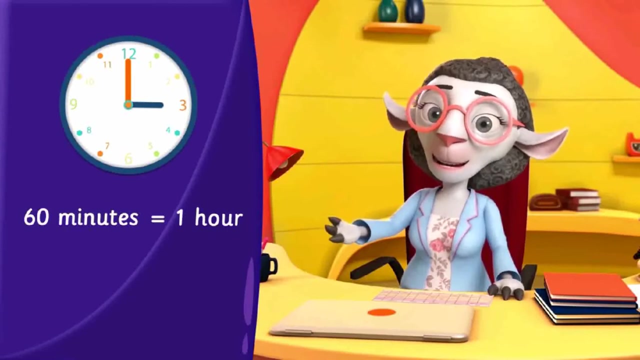 To be continued: 3 pm. Now how do we write 3.30 in words? Tap on the right answer. We know that 60 minutes is equal to 1 hour and that 30 minutes is half of 60 minutes. 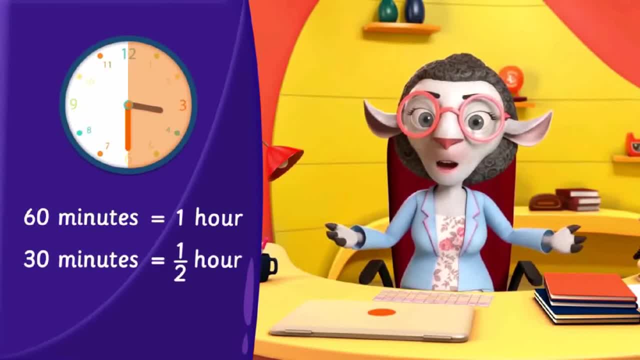 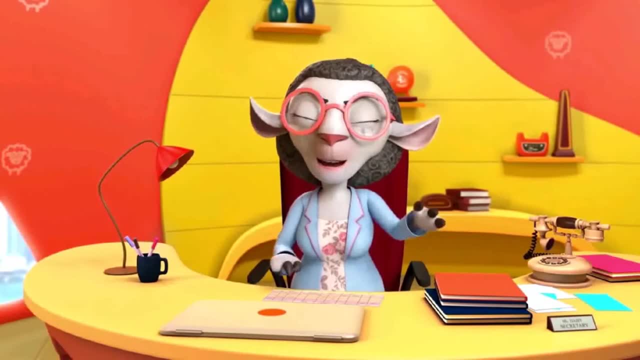 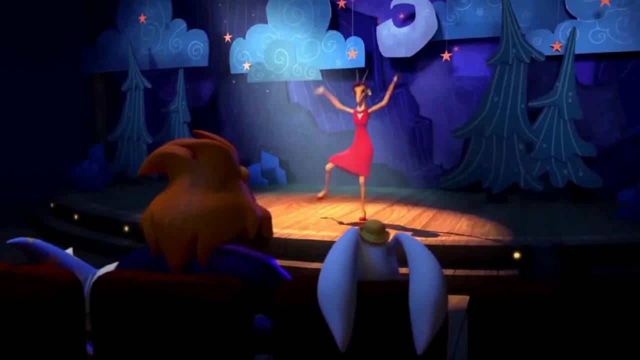 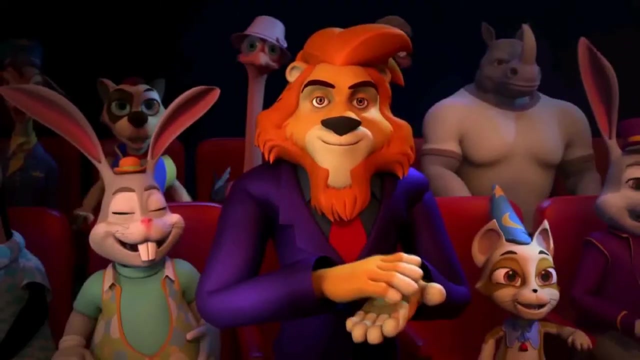 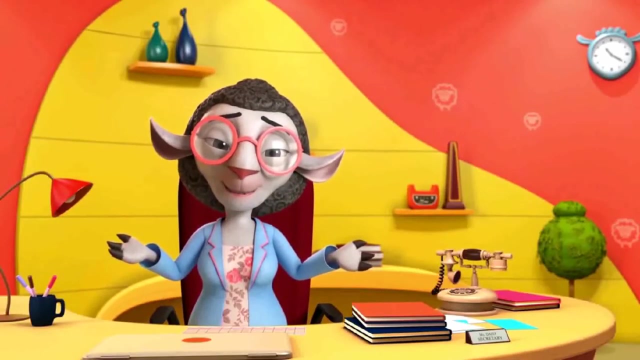 This means that 30 minutes can be written as half an hour. So we can write 3.30 as half past 3.. What Wait a second? Mr Johnny is taking ballet lessons. Well, let's move on. Let's see what Mr Johnny has to do on Thursday this week. 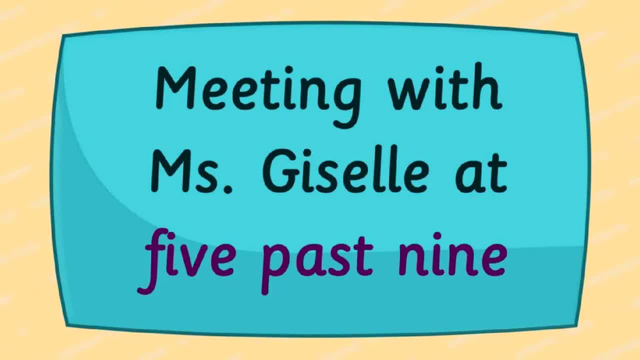 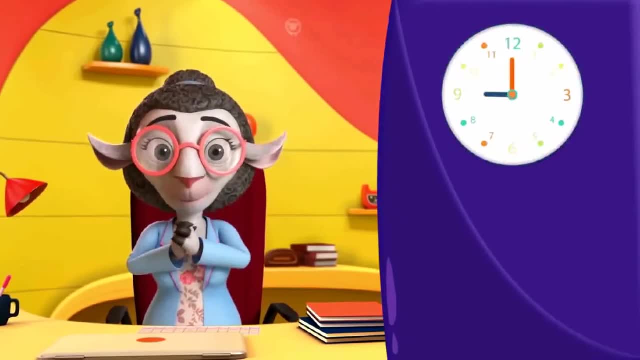 He has a meeting with Miss Giselle Again At 5 past 9 in the morning. Do you know how to write 5 past 9 in numbers? 5 past 9 means it's 5 minutes past 9 o'clock. 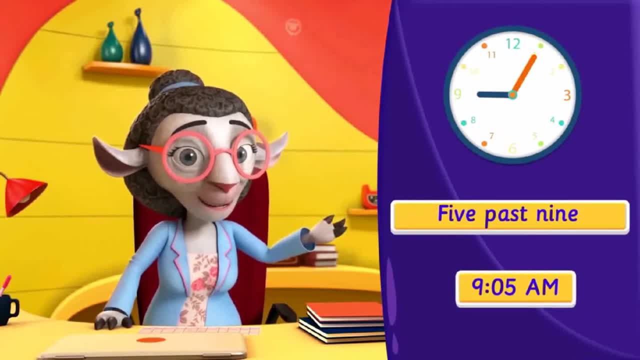 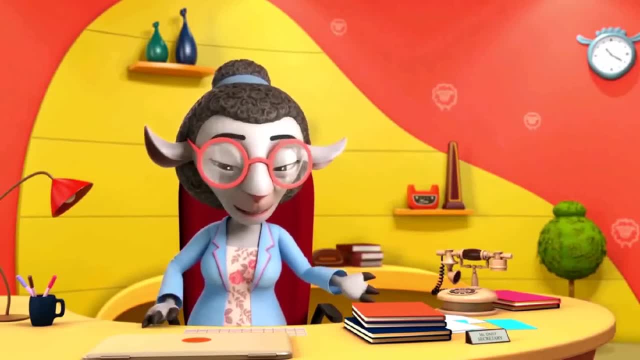 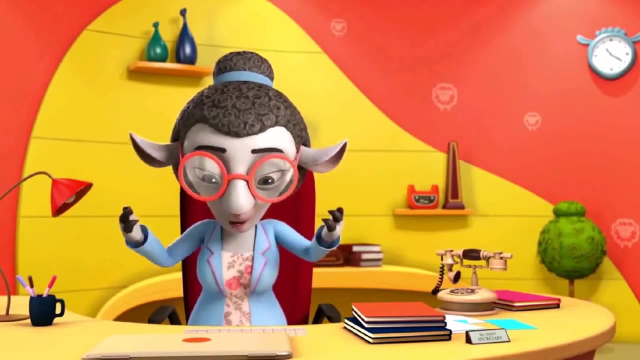 So we can write it as 9.05 am. All right. Finally, let's move to the next day, The last one. The last working day of the week is Friday. Let's see what Mr Johnny is doing on Friday. 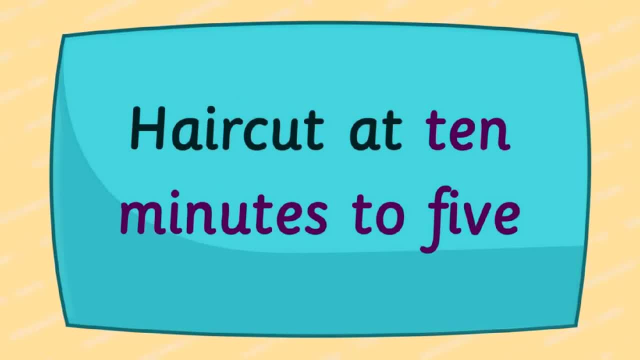 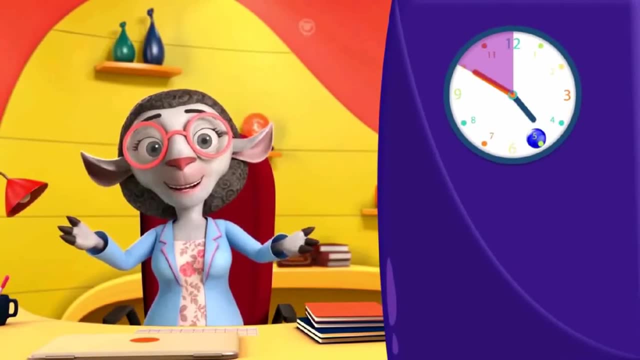 He has to get a haircut done at 10 minutes to 5 in the evening. Hmm, 10 minutes to 5 means that we're 10 minutes behind 5 o'clock, Because between 4 o'clock and 5 o'clock there is 1 hour, which means there are 60 minutes.